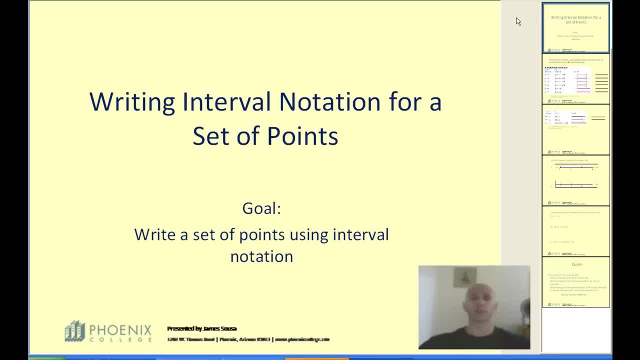 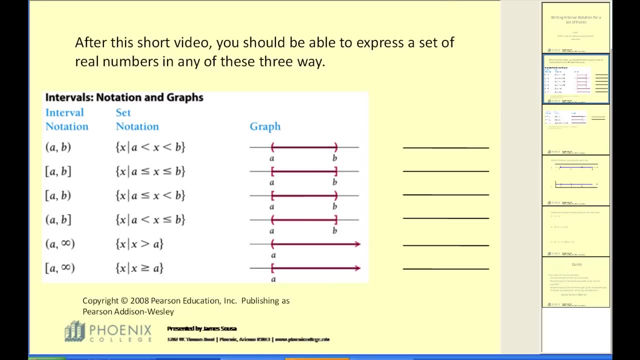 Writing Interval Notation. Our goal today is to write sets of points using interval notation. We've already written sets of points by using graphs and inequalities, but today we want to learn how to do it using something called interval notation, And once you learn it, I think you'll like it. 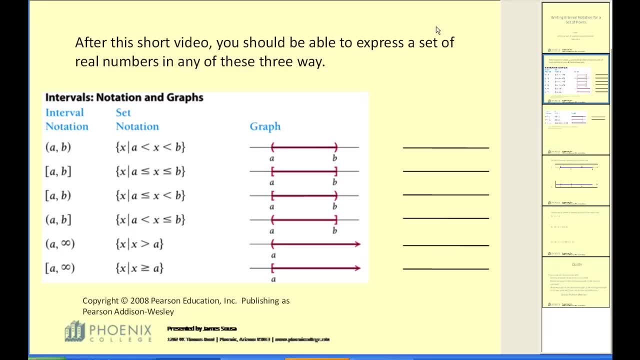 Let's go ahead and take a look at the definition of interval notation. Now, this looks a little busy. What I'd like you to do is focus in on the second column, And the second column is called set notation, And the way you read this, you would say x, such that a is less than x less than b. 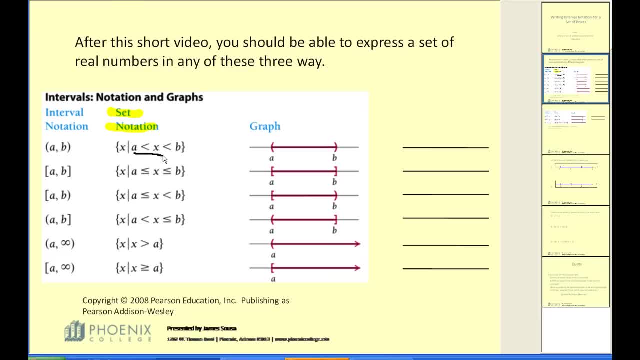 And again, what I want to focus on is this: inequality here compound inequality, And you can see that x is less than b and x is greater than a. The graph of this, from what you're probably used to seeing, would be something like this: 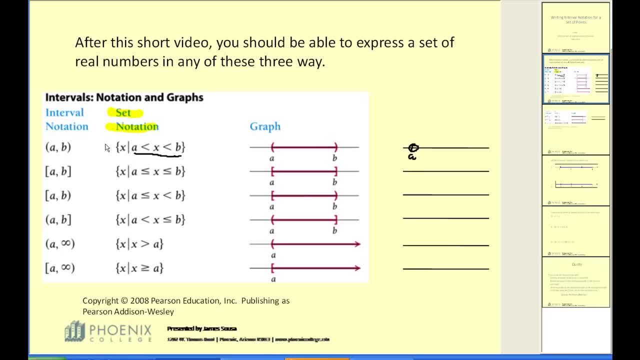 Where the value of a is on the left, it's an open circle Because of the inequality symbol. B is on the right, It's also an open circle Because of the inequality symbol, And it's the interval between those often called an open interval. 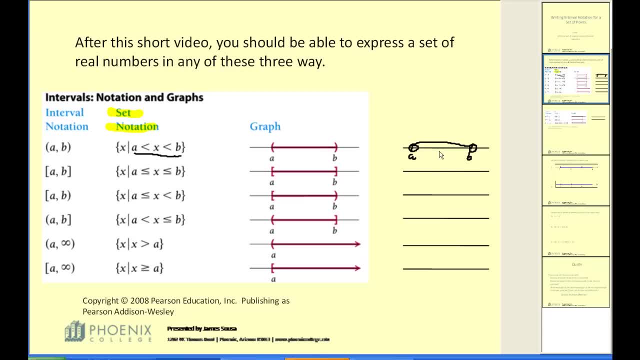 Because these are open points. Now, another way to express this same graph: instead of using open points, you can use parentheses or rounded parentheses. Those mean exactly the same thing. The nice thing about this is, once you have the graph, it makes an easy transition to interval notation. 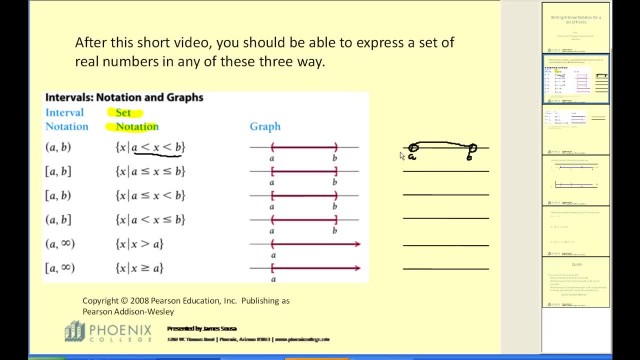 If you look on the far left, you can communicate the same information by using this notation here, Such that the interval notation a, comma b, with rounded parentheses. This is the open interval from a to b, This first column, second column, third column and fourth column. 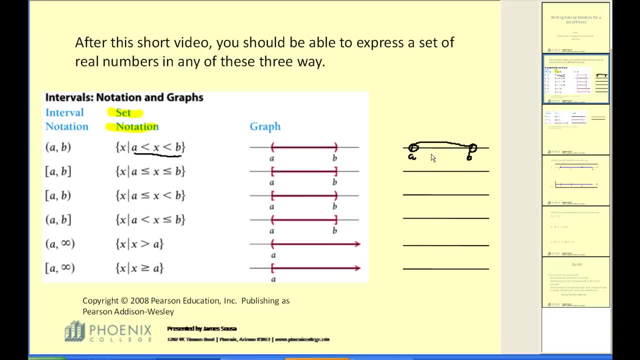 all communicate the same information in a different way. If you look at the next row here, the only difference here is this is the closed interval, Because the values of a and b are included in the interval. So this graph would look very similar to the first. 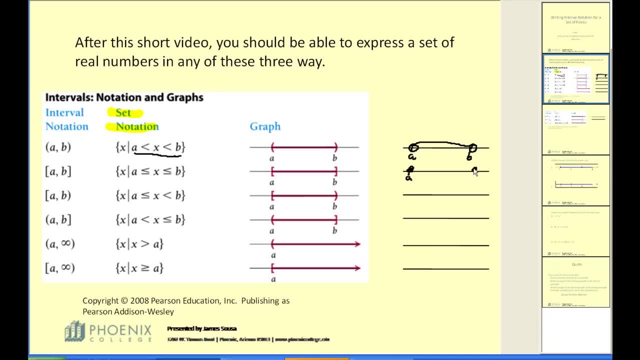 Except at a you'd have a closed point, And at b you'd have a closed point as well. So what you can get from this is that closed points are the same thing as a square bracket. These two graphs are equivalent. 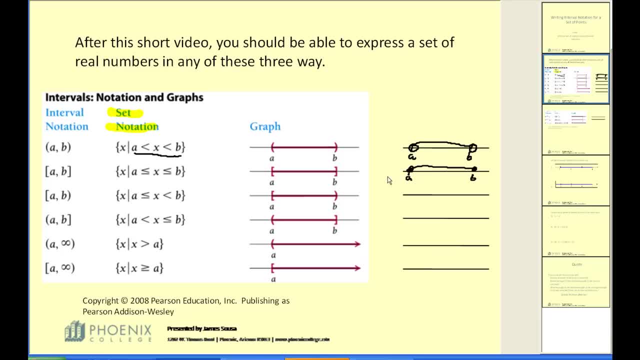 Again, once you have this graph, it makes a nice easy transition to interval notation. The closed interval from a to b can be expressed in this manner: a comma b with both ends as square brackets. Now these next two I won't graph. 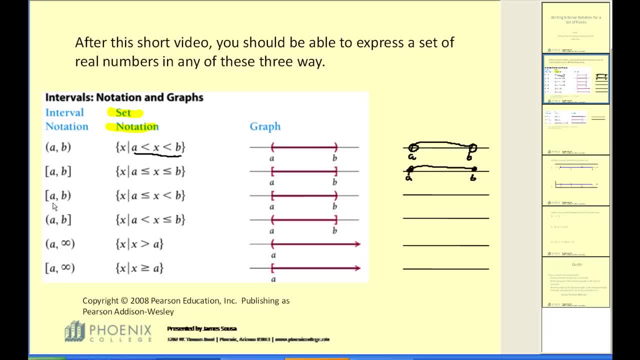 but you can see, this is just a combination where this is what you would call a closed interval at a and open at b, And the next row open at a and closed at b, Just meaning, for example, in this case it would have an open circle or open point at a. 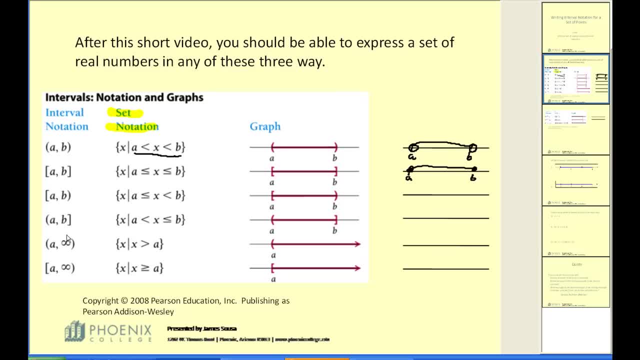 or a closed point at b. Let's skip down to this next example. Again, I want to kind of make the connection between this inequality here, The way you would read this again: x, such that x is greater than a. Let's graph that. 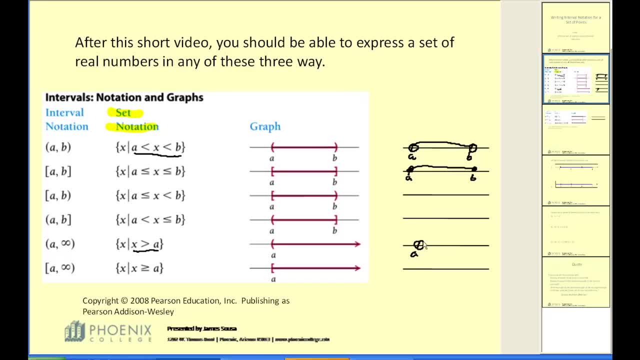 We'd have an open point at a, and greater than a would go to the right. Now, if you go to the right of the number line, you are going to approach positive infinity, And I like to add that in. there Again, the only difference between these two graphs. 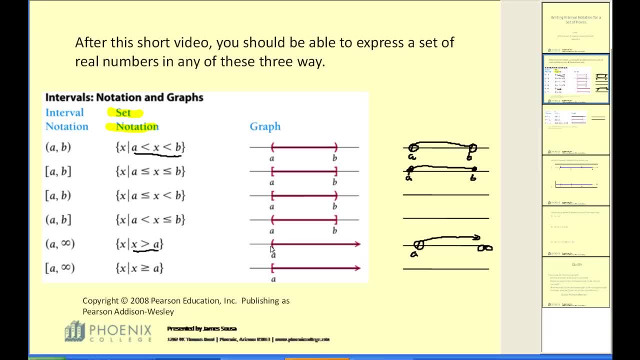 this is using an open point and this is using a rounded parenthesis. However, once you have the graph, if you take a look at this graph and you jump all the way to the left to interval notation notice, there's the a. 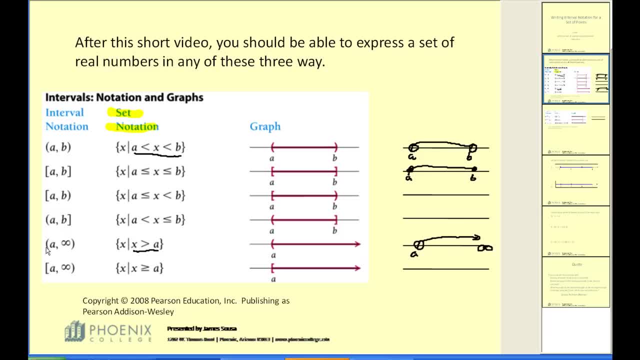 there's the infinity. now there's rounded parenthesis, a because of the open point, And if you have an infinity or negative infinity in interval notation, you're always going to use the rounded parenthesis because, technically, infinity and negative infinity do not exist. 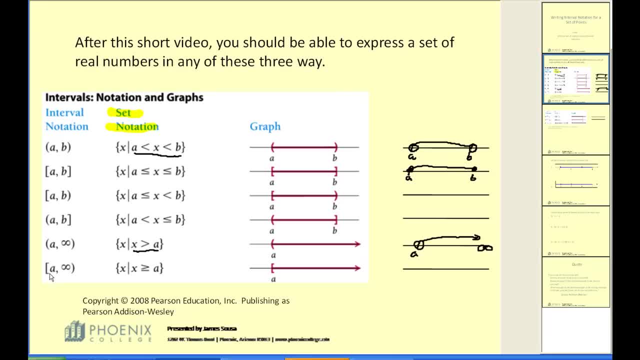 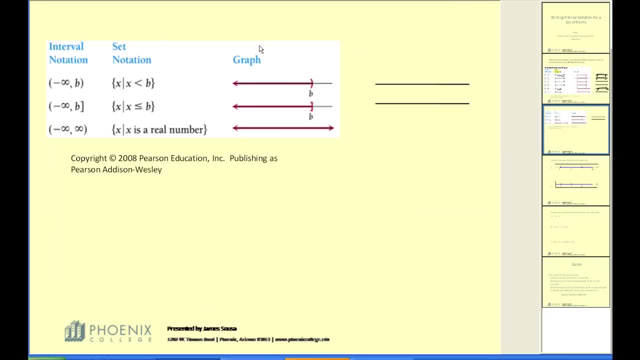 The only difference between this next row is that it's closed on a. So we have the square bracket. Let's look at a couple more examples here, or definitions: Notice on this graph. this would correspond to an open point. I won't graph it. 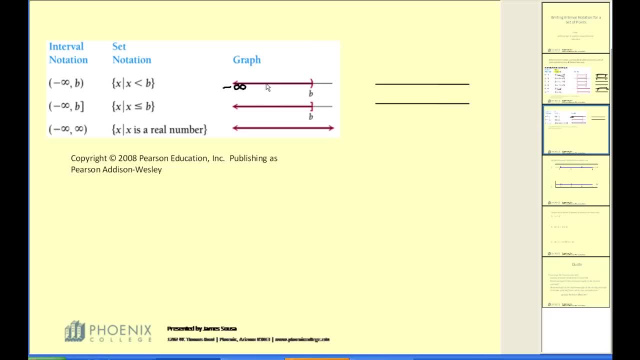 And if you go to the left you are approaching negative infinity. So, as you can see from the far left, the interval notation negative infinity to b, both with open parenthesis. The last example here, if you're graphing numbers on the number line, 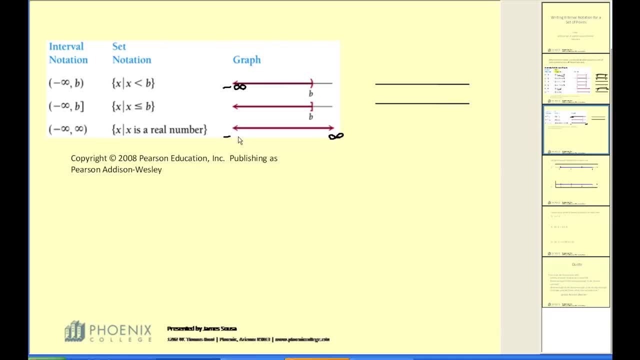 of course, in the direction- positive direction- you have positive infinity, negative direction, negative infinity. and that's where this interval notation comes from. It's the graph of all real numbers. Let's take a look at some specific examples. Write the interval notation for each set. 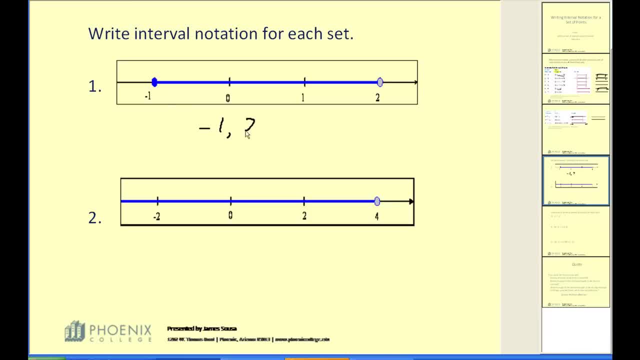 This interval starts at negative one, goes to positive two. It includes negative one, so that means we have to write or use a square bracket. It does not include two, so it would use a rounded parenthesis. This next example, as you can see, 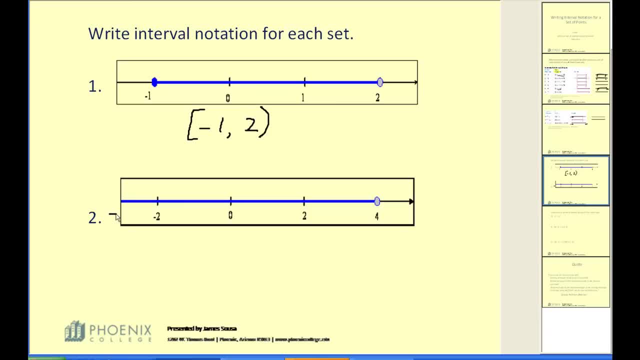 the graph goes left forever. That approaches negative infinity Again. I like to include that because it helps me make the transition to interval notation. Interval notation for this interval would be from negative infinity to positive four, Negative four and, of course, always open on negative infinity. 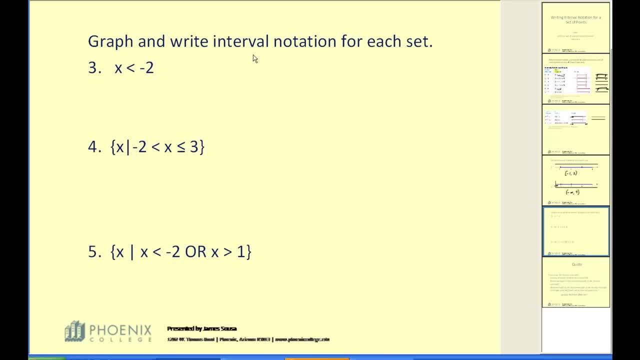 A couple more. Now we want to graph and write interval notation for each set. So let's graph: X is less than negative two. It'd be an open circle and arrow to the left. That's really all that I need, but I do like to include again. 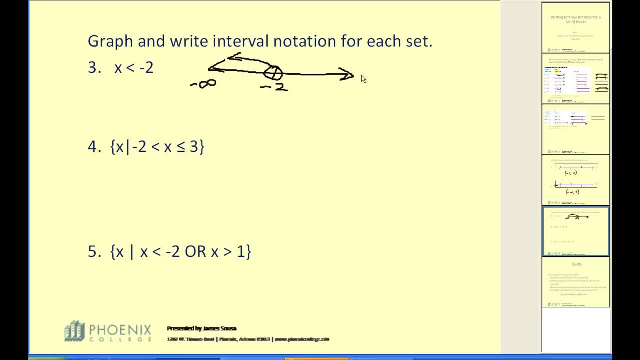 the negative infinity. going to the left, Interval notation would be from negative infinity to negative two and it would be open on both. Two more here and we'll be done X, such that negative two is less than X, less than or equal to three. 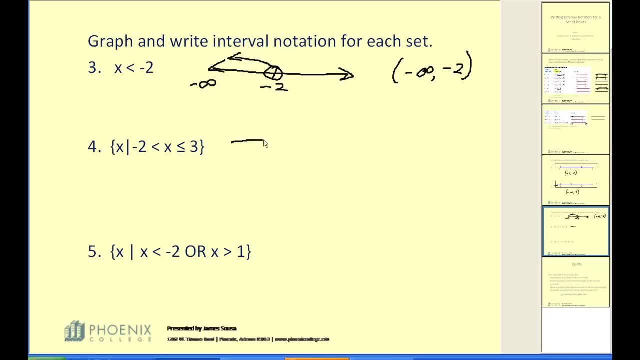 Have a compound inequality here. Let's go ahead and graph it. X is kind of sandwiched between negative two and positive three. It does not include negative two but it does include positive three and the interval is between those. Interval notation for this.